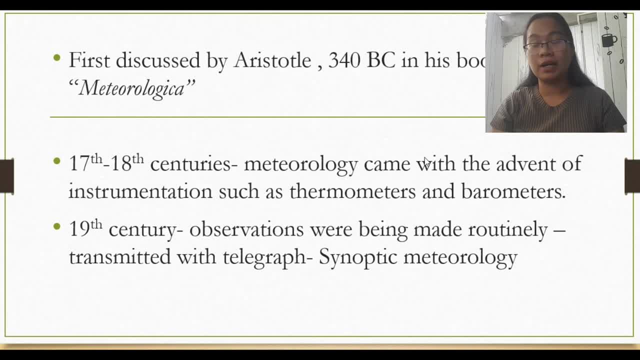 But during the 17th and 18th centuries there were instruments like thermometers to measure the temperature and then barometers to measure pressure. In the 19th century we are having the observations being done. It is being done routinely, and then it is also being transmitted with telegraph. that is what we call synoptic or synoptic meteorology. 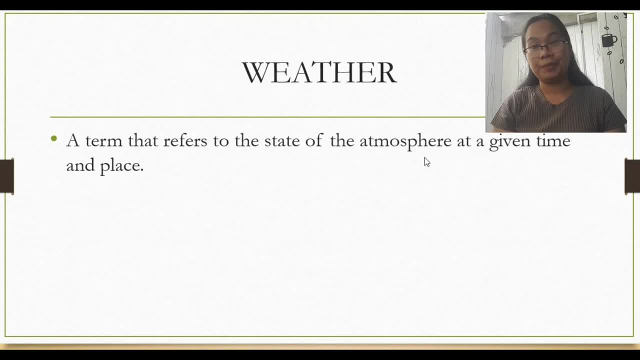 Okay, how do we define weather and how is it different from climate? The term weather refers to the state of the atmosphere at a given time and at a given place. It may actually change. for example, within the day, we may have different weather conditions. 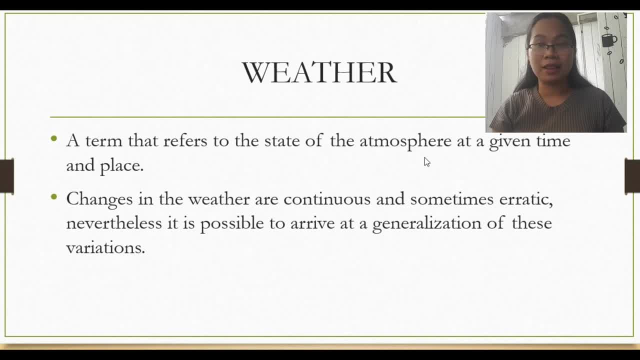 Okay, The weather conditions are also different. Within the month, we have different weather conditions. Changes in the weather are continuous and sometimes erratic. Nevertheless, it is still possible to arrive at generalization of these variations. So that is how we define weather. 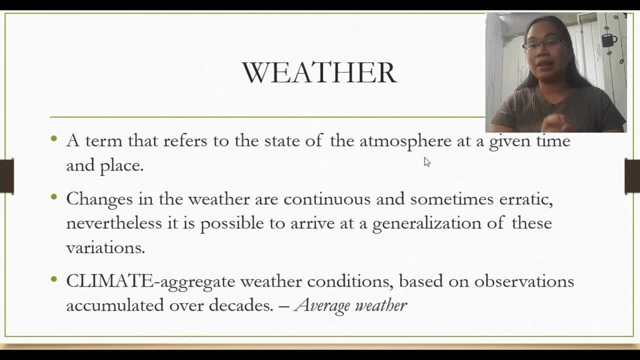 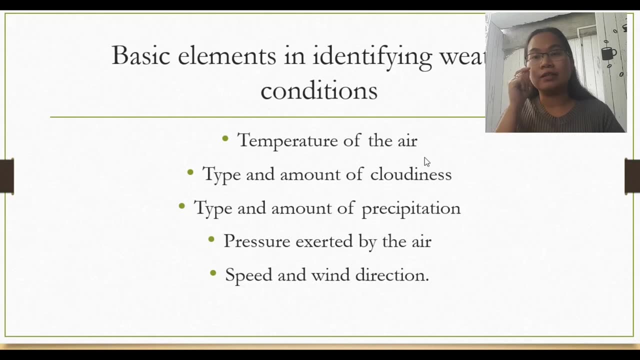 It is different from climate because climate is an aggregate weather conditions based on observations which were accumulated over decades. There are basic elements for us to be able to identify weather conditions. In meteorology. we have to describe the temperature of the air, the type and amount of cloudiness, the type and amount of precipitation, the pressure exerted by the air and the speed and wind direction. 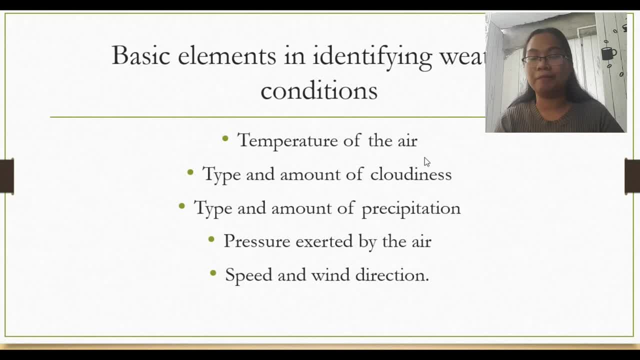 In our course meteorology. we are going to cover that chapter by chapter, So it is not yet part of the introduction. But as we go along the discussion of weather conditions In the course of meteorology we will be able to identify those weather conditions. 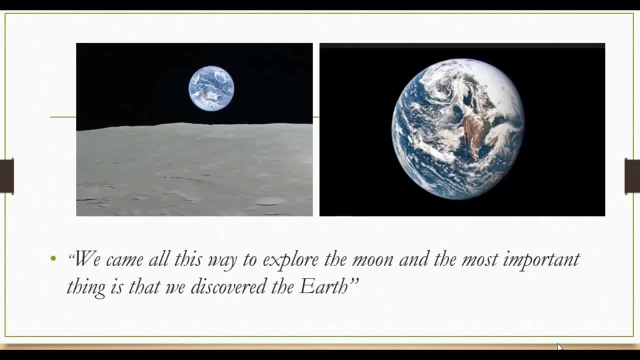 The first photograph is the Earthrise and then the other one is the Blue Marble, Where, in Earthrise, it was resulted from the exploration of Apollo 8, and then the Blue Marble by Apollo 17.. They were trying to understand the Moon and that exploration was to explore the Moon. 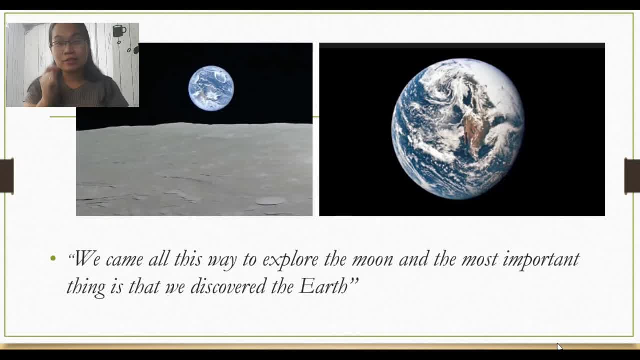 But they were able to understand the Earth better because of that exploration. They were able to see the atmosphere of the Earth: There are swirling clouds, and then it is considered as a blue planet, and so on. So that's why we have here the quotation: we came all this way to explore the Moon. 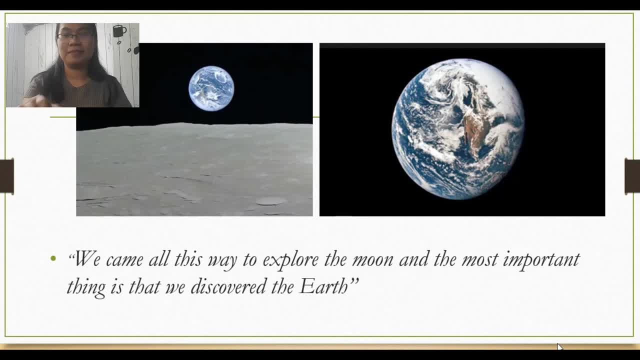 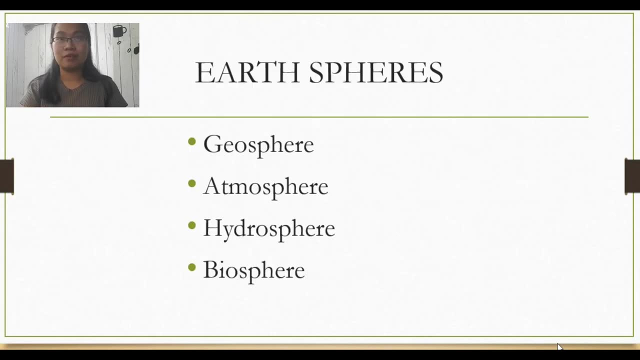 And the most important thing is that we discovered the Earth. So in this course, also in this course, you are going to discover more about the Earth. You are going to understand our home planet Earth. I think you are able to discuss this in your Earth science. 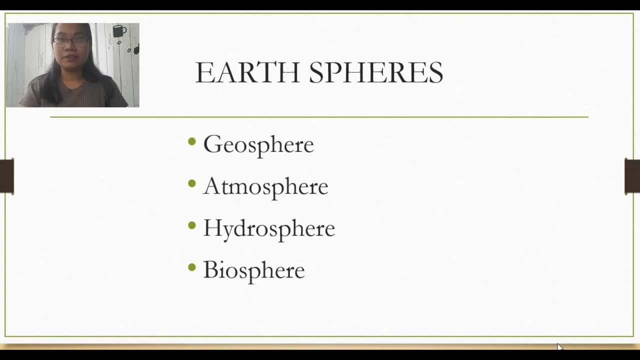 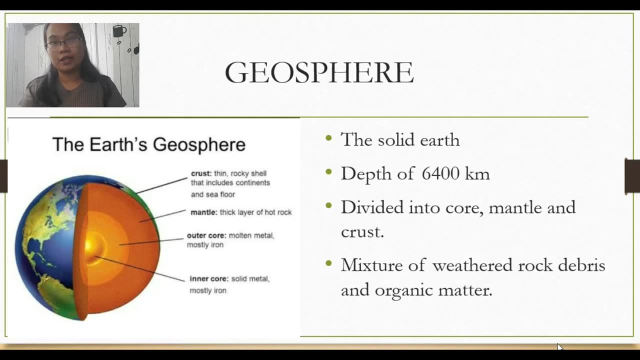 We have the Earth spheres, We have the Geosphere, the Atmosphere, Hydrosphere and Biosphere. Geosphere- from the term Geo, that is, the solid portion of the Earth. It has a depth of around 6400 kilometers. 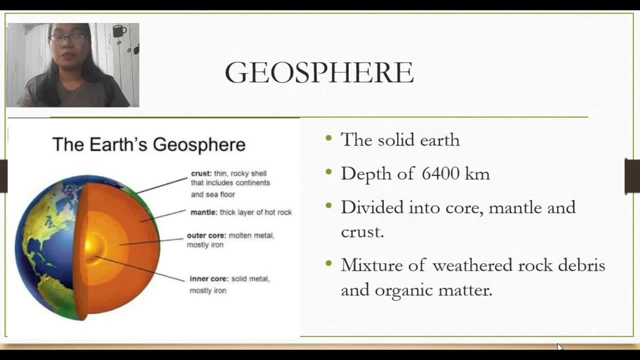 It is divided into core, mantle and crust. As we know the crust, that's the thinnest. It is a portion of the Earth's Geosphere. And then we have the mantle, the thick layer of hot rock. Then we also have the outer core, made up of molten metal, mostly iron. 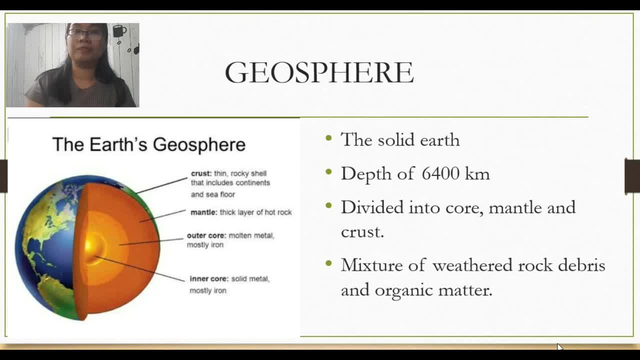 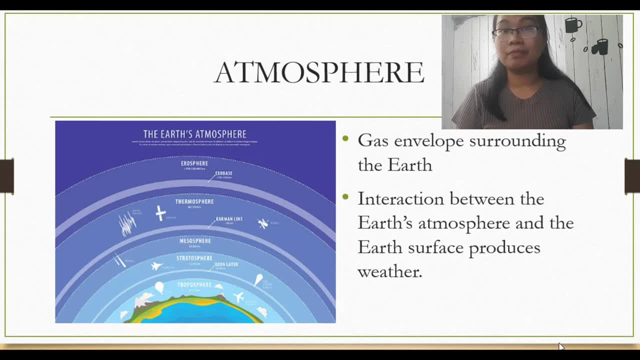 And the inner core, solid metal and also mostly iron. The Atmosphere: it's the gas envelope surrounding the Earth. We have an interaction between Earth's Atmosphere, and the Earth's surface produces weather, So all weather conditions that we have, of course, can be found in the Atmosphere. 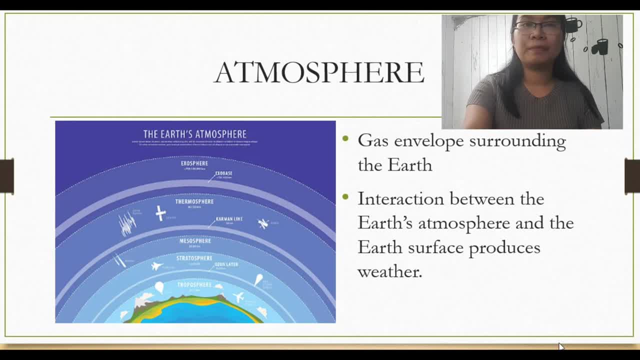 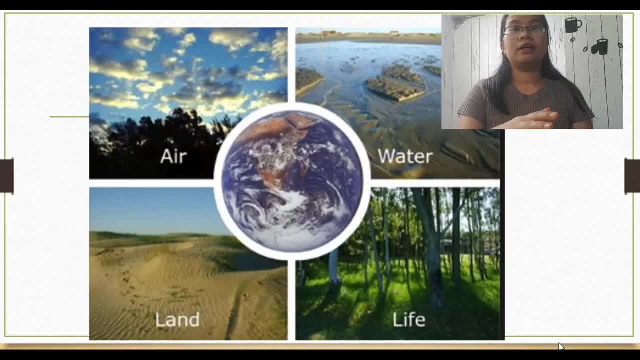 But it is also affected by the Geosphere. Later we are going to discuss the different layers of the Atmosphere. There we have the Air, Water, Land and Life. Those are the four spheres of the Earth. We have the Air so that it represents the Atmosphere. 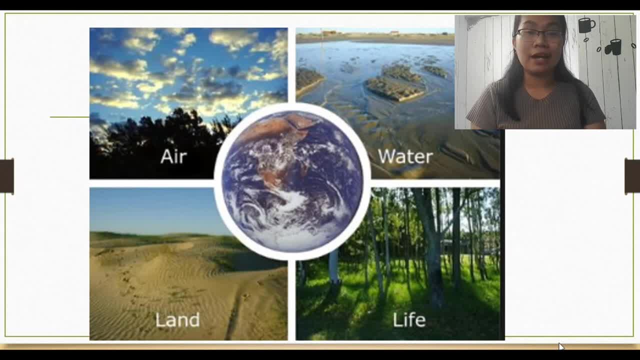 And then the Water, we have the Hydrosphere, the Land, the Geosphere, and then the Life is the Biosphere. So they are all interrelated. That's why we consider them as a system or as the Earth system. One sphere can affect the other and it can have an effect on all parts of the Earth system. 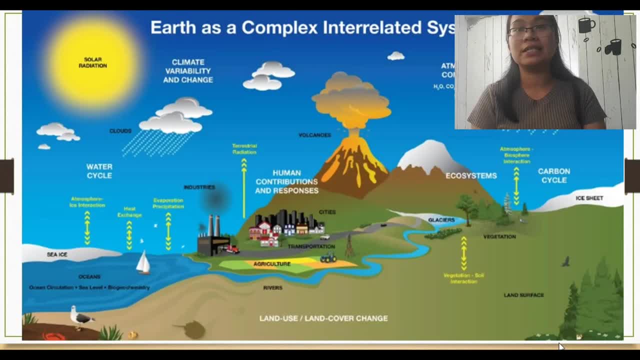 For example, we have here Earth as a complex interrelated system, So water cycle, which deals with the Hydrosphere and the Atmosphere. there is an interaction between the Hydrosphere and the Atmosphere When water vapor or when water evaporates. 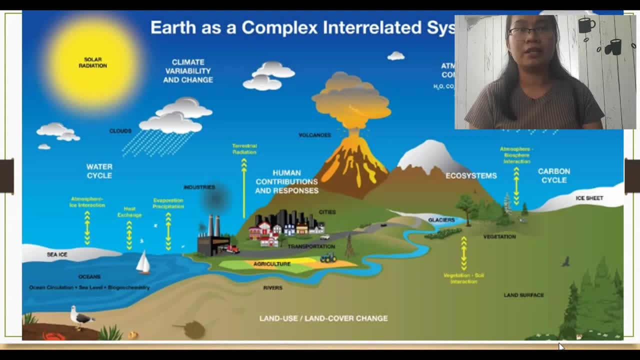 water from oceans or different bodies of water. they evaporate and then it will go through the Atmosphere and they have an interaction And then of course even the Biosphere can affect that. Even the Biosphere can be affected, For example, if we have weather conditions. 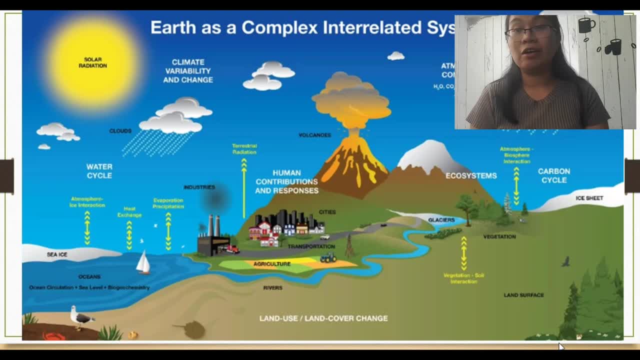 if the rain is strong, there will be rain, So it may cause landslides, So that will affect the Geosphere, Or that has affected the Geosphere, And then it can have damage to the lives of people, So that will affect the Biosphere. 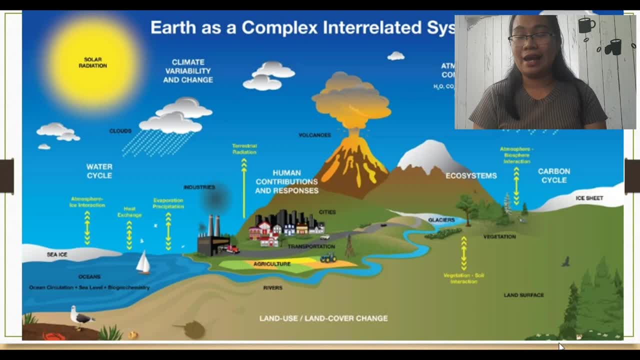 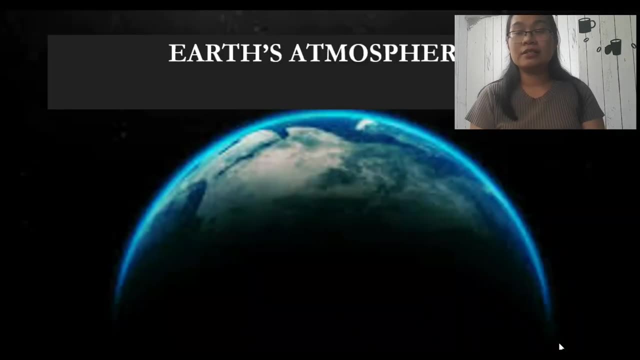 So they are all interrelated: The Ecosystems, the Atmosphere, the Geosphere, the Hydrosphere, the Biosphere. they are all connected, So that's why we consider them as the Earth System. Now let's discuss more of the Earth's Atmosphere. 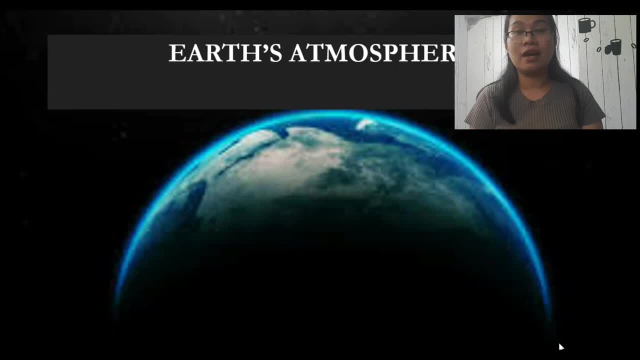 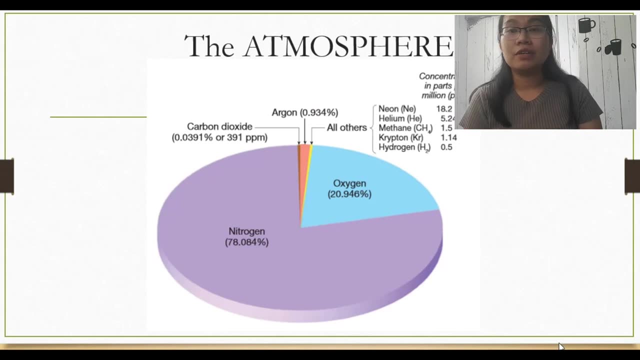 So you can see in the illustration, there's a thin layer of the air covering the Earth. So that is our Atmosphere. Now I want you to look at the composition of the gas in the Atmosphere. We have Nitrogen, which is 78.084%. 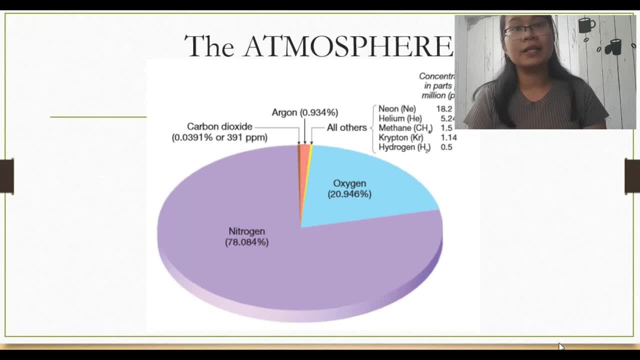 We have the Oxygen, which is 20.95%, The Carbon Dioxide, which is very small- 0.0391%. Then we have the Argon- 0.934%, And others such as Neon, Helium, Methane, Krypton and Hydrogen. 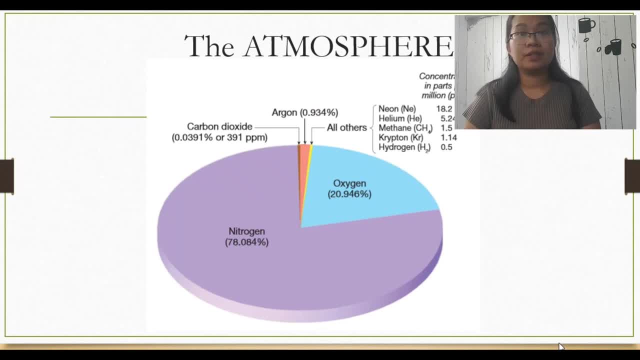 So what can you say about the gas concentration in the Atmosphere? So we still have higher Oxygen, But we know the condition of the Earth. We have what we call Global Warming. So which is It was resulted from excessive Carbon Dioxide present in the Atmosphere. 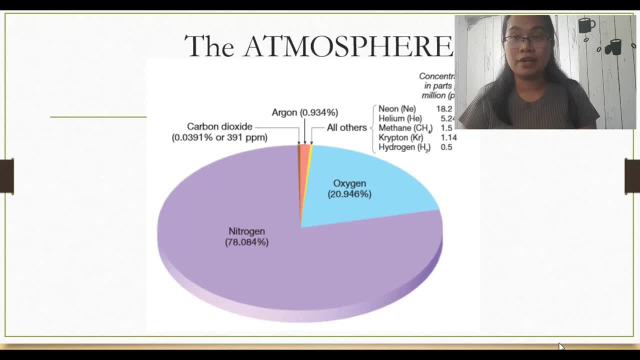 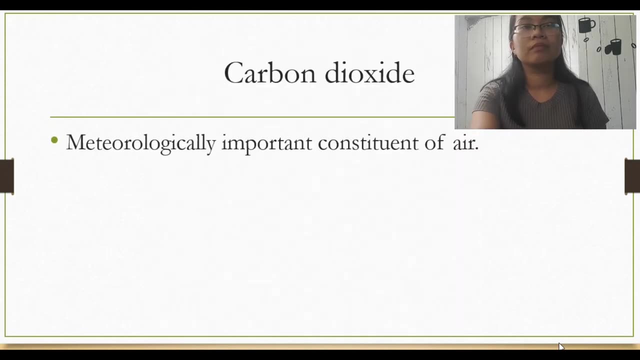 So that is another way that we interact with the Atmosphere, The Biosphere producing a lot of Carbon Dioxide which may affect the Atmosphere or our weather conditions. Let's discuss the gases one by one. Let's first have Carbon Dioxide. 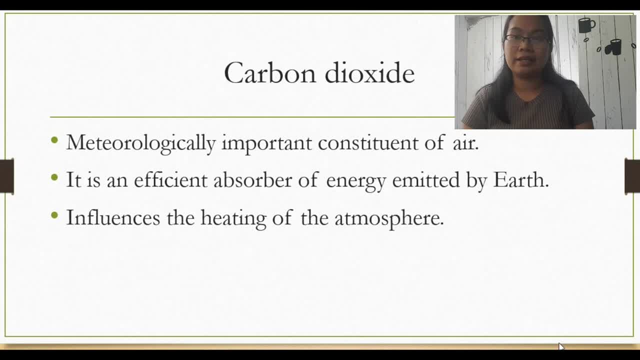 Carbon Dioxide. even though its amount is small in the Atmosphere, it plays a major role in the weather conditions that we have. It is considered as meteorologically important constituent of air because it is an efficient absorber of energy emitted by the Earth. 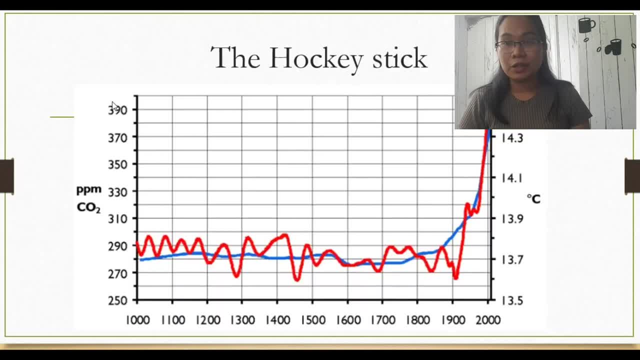 Okay, again, the Earth receives solar radiation, or solar energy coming from the Sun, But it also radiates that energy, And then that energy could be trapped in the Atmosphere because of the presence of Carbon Dioxide. This Carbon Dioxide, even though they are only a portion or a very small amount in the Atmosphere, 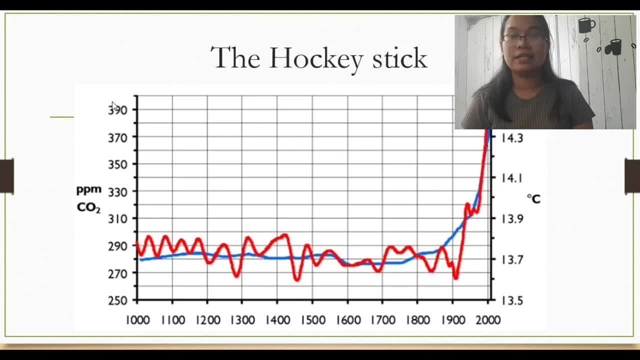 they are a very efficient absorber of the heat coming from the Sun and also emitted by the Earth. So you can see here in the graph we have this, what we call the hockey stick. At first, our Carbon Dioxide. we have here this level only. 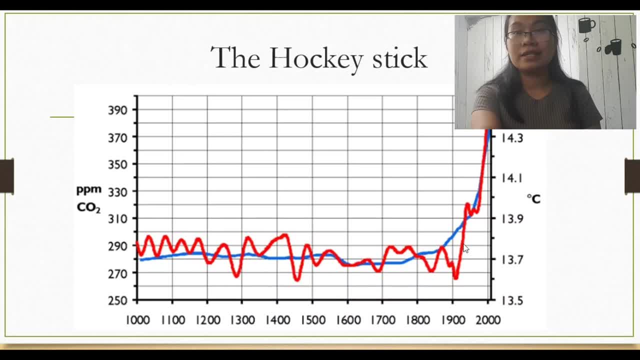 But at this point there is an abrupt change in the level of the Carbon Dioxide present in the Atmosphere. Now, did you remember the news before that, when there was a lockdown, according to scientists, we also had a decrease in the level of Carbon Dioxide. 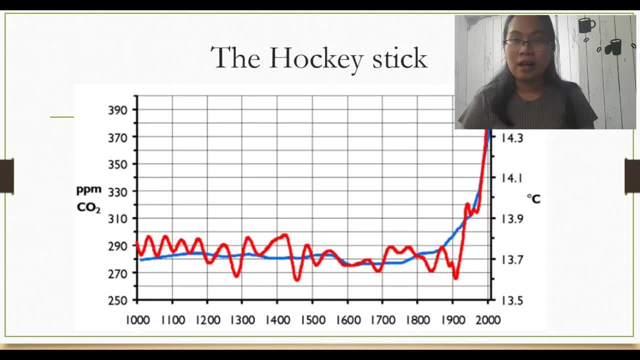 So what could be the reason behind having a Carbon Dioxide concentration increased, Higher concentration of Carbon Dioxide? we can attribute that to industrial activities And right now I think this could be attributed to transportation. That is why they say during the lockdown there is not much use of transportation. 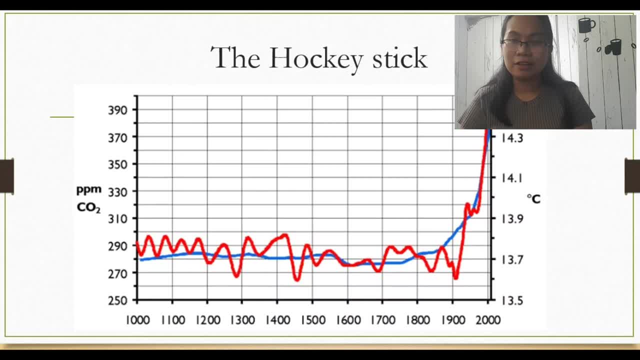 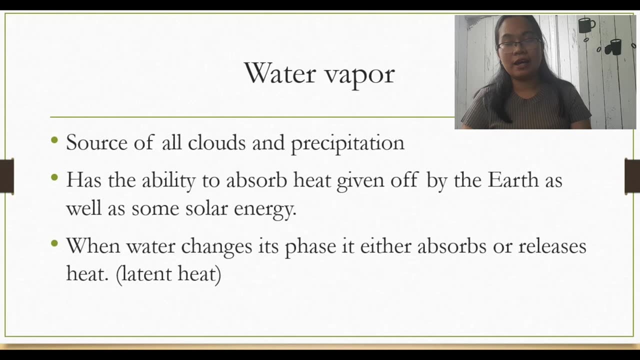 So the level of Carbon Dioxide decreased And that could be a good research for this. For this course, you can check the level of Carbon Dioxide when we had a lockdown. Another gas present in the Atmosphere. we have here water in the form of gas. 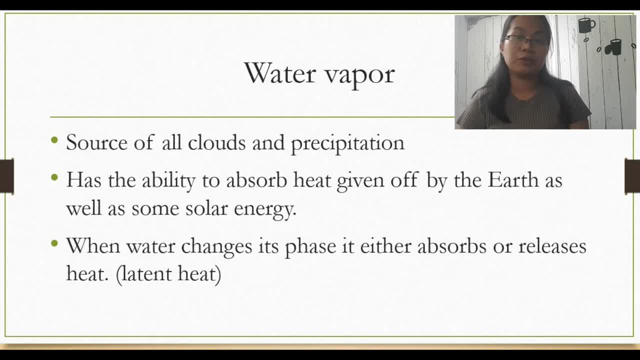 We have water vapor, which also plays a very important role in atmospheric conditions or in weather conditions. Water vapor is described as source of all clouds and precipitation, And also it has the ability to absorb heat given off by the Earth, as well as some solar energy. 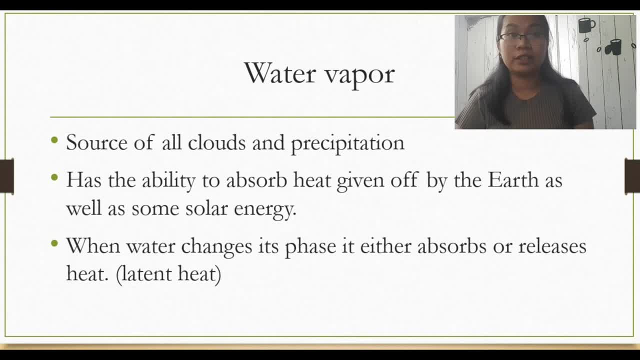 So water vapor is also a very efficient absorber of heat. When water also changes its phase, it can absorb or release heat. When we say it's absorbing heat, it could actually be considered as a cooling process for the environment. So again, it may absorb heat. 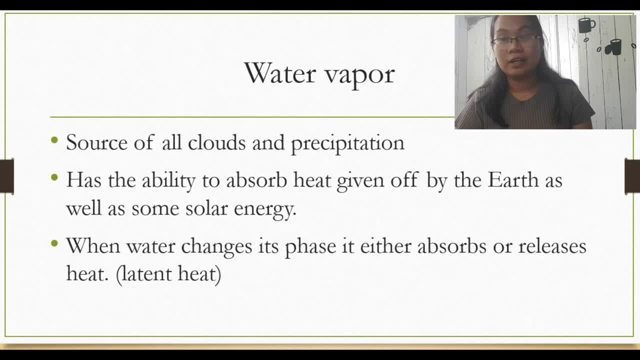 So the environment, that it will leave energy. the temperature will decrease, But also, during a phase change, it may also release energy, So there will be an increase in temperature in the surroundings. So you see, water vapor will really play a big role in our climate or in our weather conditions. 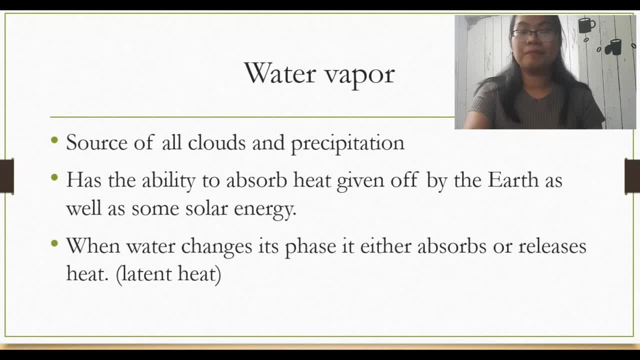 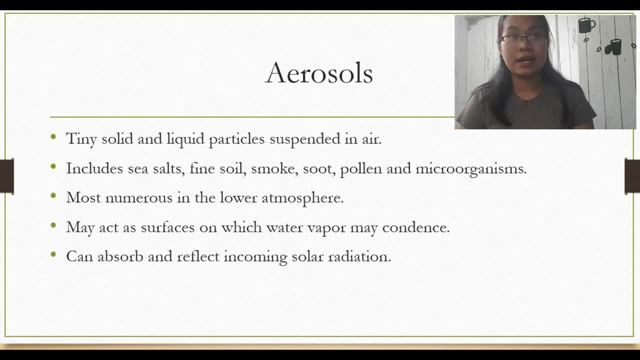 Up and down temperature. Okay, We have aerosols. They are tiny solids and liquid particles suspended in air. It includes sea salts, fine soil, smoke, soot, pollen and microorganisms. They are also most numerous in the lower atmosphere. 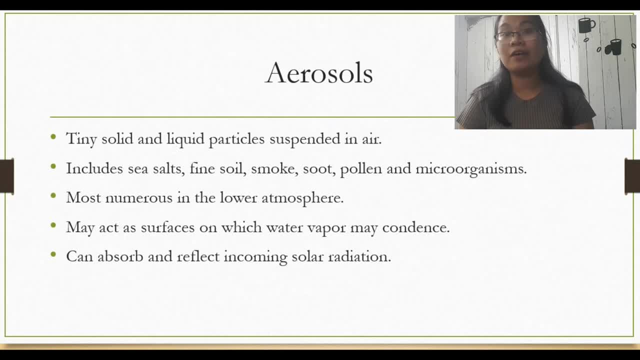 And they may act as surfaces on which water vapor may condense during the process of condensation, before it rains. So aerosols also play an important role for our weather conditions. They can absorb also and reflect incoming solar radiation, Okay, And they contribute to optical phenomena. 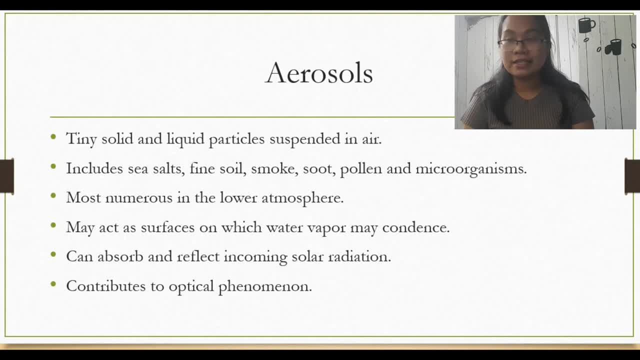 For example, why is the sky red during sunset? Why is the color of the sky different when we are in Metro Manila? Because there are larger suspended particles there compared to when we are in the province or Zambales, So they contribute in that optical phenomena. 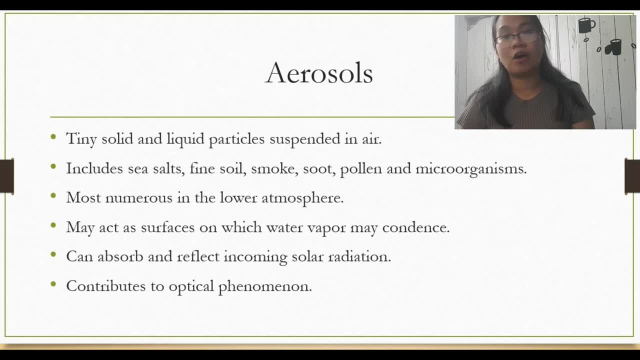 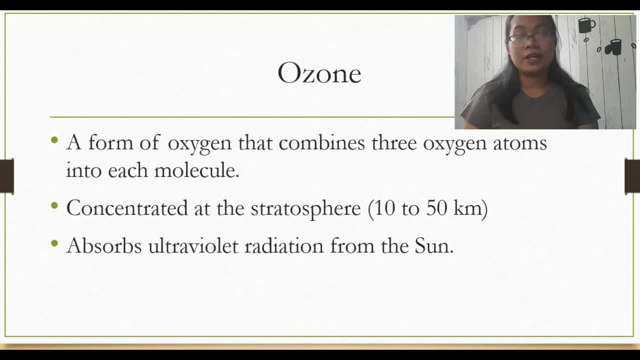 Hopefully we can reach that discussion on optical phenomena also. And then another gas which plays an important role in the atmosphere is ozone. It is a form of oxygen that combines three oxygen atoms into each molecule. This ozone is concentrated in the stratosphere. 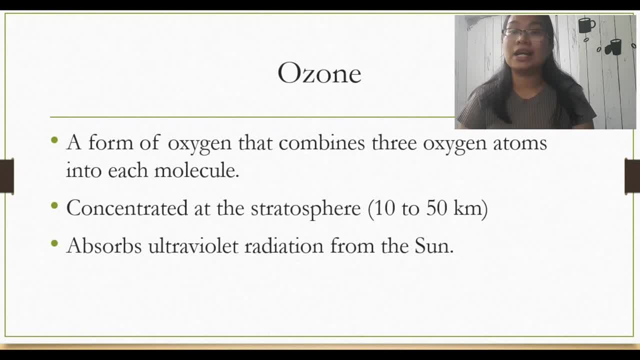 That's why they say ozone layer is found in the stratosphere. They are also considered to be absorbent of ultraviolet radiation coming from the sun. That's why, when they say ozone layer depletion occurs, there will also be higher solar energy that will be absorbed by the earth. 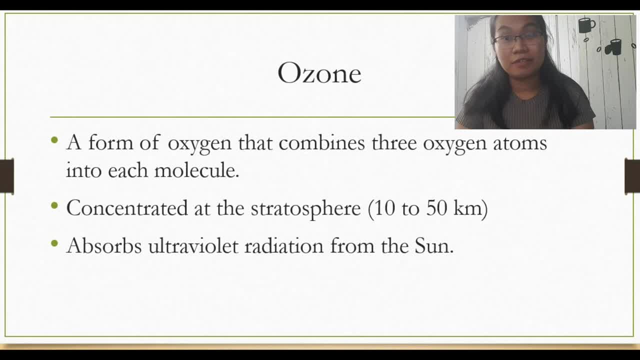 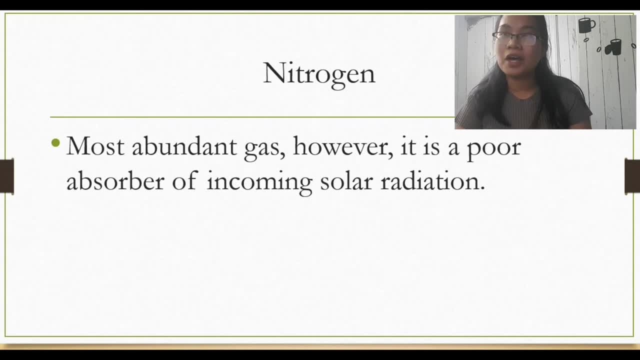 specifically UV rays, especially ultraviolet radiation, which is very harmful for us. Nitrogen is also a gas. It is the most abundant. However, its contribution is small when it comes to weather conditions because it is considered to be a poor absorber of incoming solar radiation. 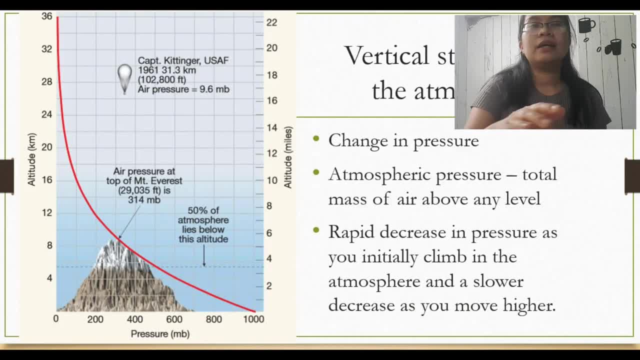 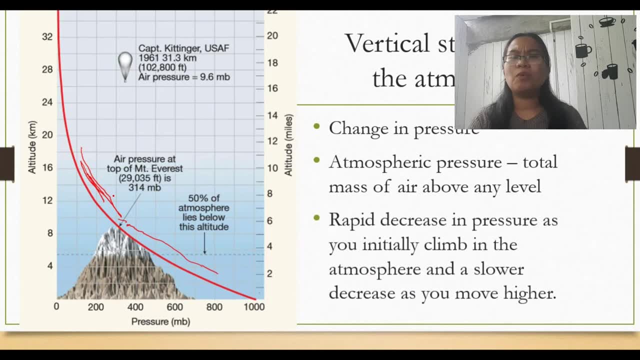 Okay, now I want you to look at this one: The vertical structure of the atmosphere. Okay, so what is pressure? Atmospheric pressure is the total mass of air above any level. When we say pressure, it's force per unit area In physics. when we say force, for example, 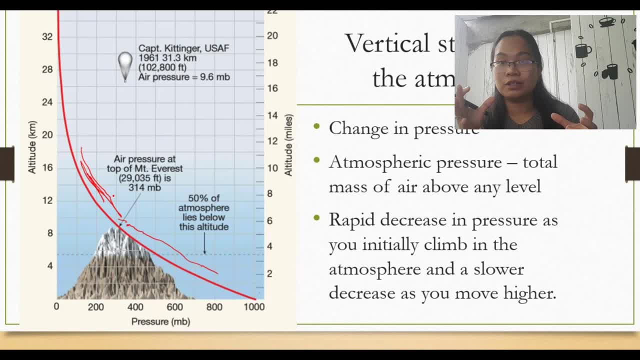 we have air. Its mass is considered to be the mass of air. You will make it a force, so that will be the weight of the air And then that is the force that it exerts at a particular area, So that is atmospheric pressure. 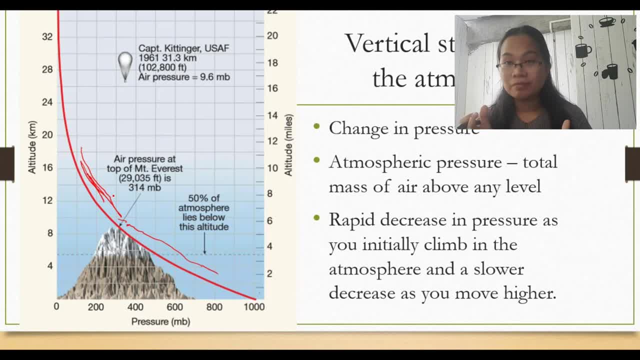 It's the weight or the force exerted by the air. So that is the air column in that particular area. You can see here, initially there is an abrupt decrease in pressure And then after that there is a gradual decrease in pressure as the altitude increases. 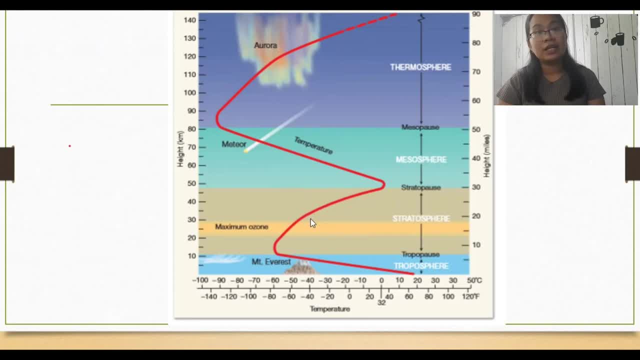 Okay, now I want you to look at this. These are different layers of the atmosphere. We have the troposphere, stratosphere, mesosphere and thermosphere. And look at how temperature changes in the different layers. You can see here in the troposphere as you go higher in the troposphere. 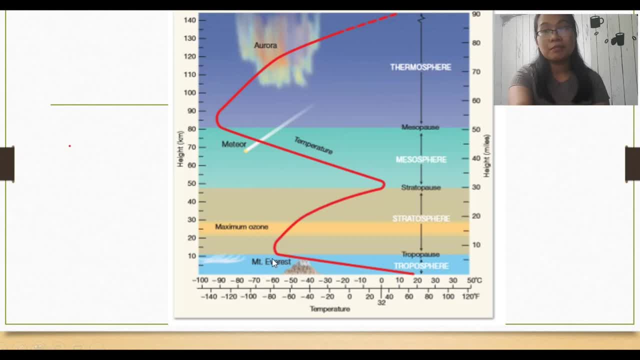 the temperature decreases. When you arrive at the stratosphere, the temperature increases When you arrive at the mesosphere, temperature decreases again, And then when you go to thermosphere, temperature increases again. Now let's describe each layer of the atmosphere. 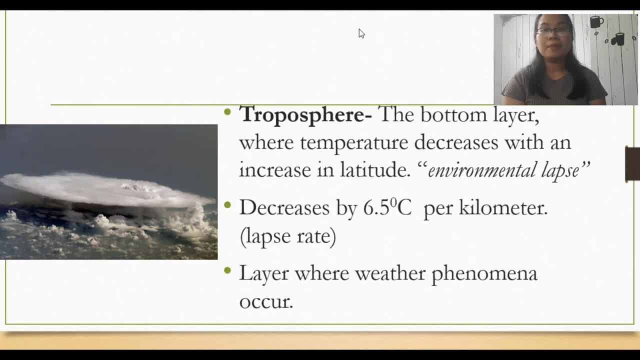 Okay, let's have first the troposphere. Troposphere is the bottom layer of the atmosphere, where temperature decreases with an increase in altitude. We have what we call environmental lapse. So how much is the decrease in the temperature? It is 6.5 degrees Celsius per kilometer. 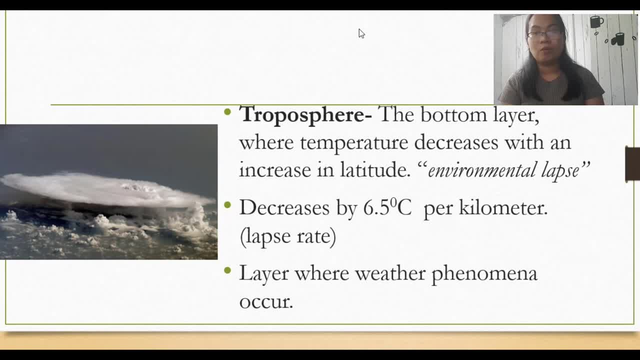 So that is the environmental lapse rate. One kilometer: it will decrease to 6.5.. Another kilometer: it will decrease to 6.5.. It is also known to be the layer where weather phenomena or weather conditions happen. Okay, also, the sphere is also known as the weather sphere. 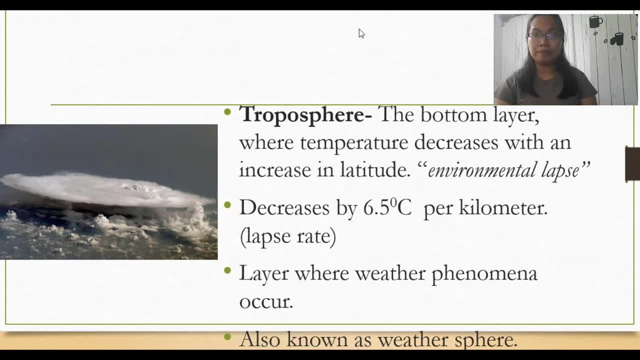 Okay, what happens to the temperature in the troposphere As you go higher in the altitude in the earlier illustration? as you go higher in its altitude, the temperature decreases because you are moving further from the Earth. As you know, Earth also releases heat. 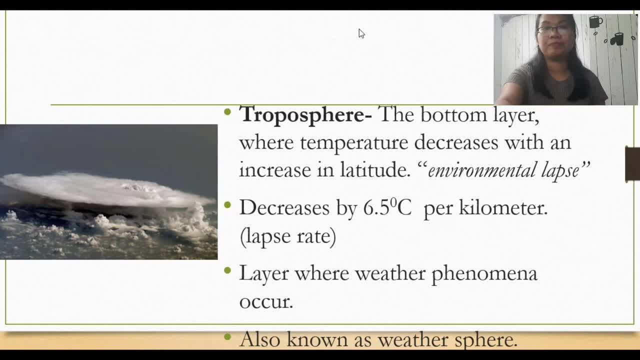 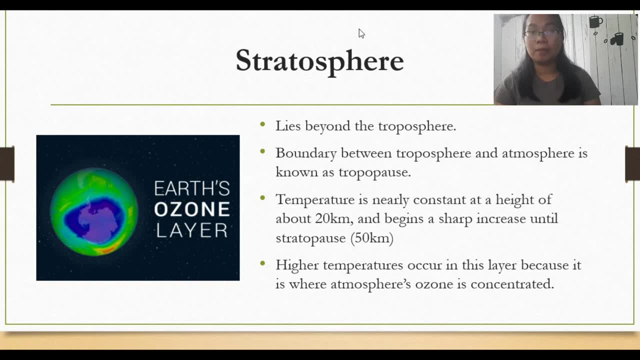 So when you get closer to it, the temperature gets colder. Next layer: Let's now discuss the stratosphere. It lies beyond troposphere. So first layer is the troposphere, The next is the stratosphere And then the boundary between troposphere and stratosphere. 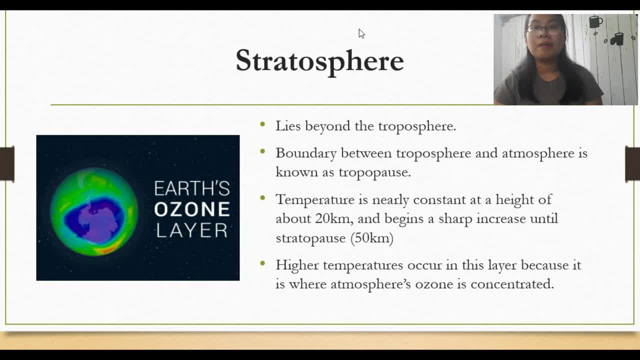 is also known as tropopause. The temperature is nearly constant at the height of about 20 kilometers and then begins a sharp increase until stratopause, which is at 50 kilometers. Higher temperature occurs in this layer because it is where ozone layer is found. 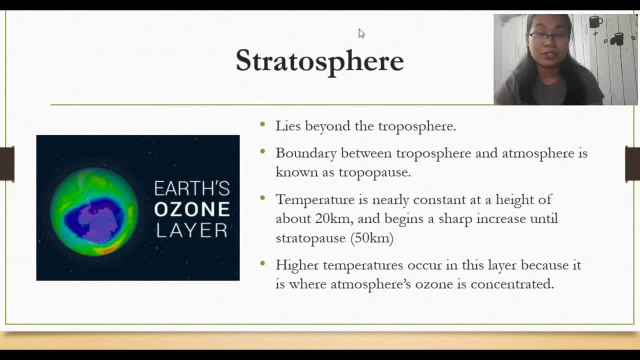 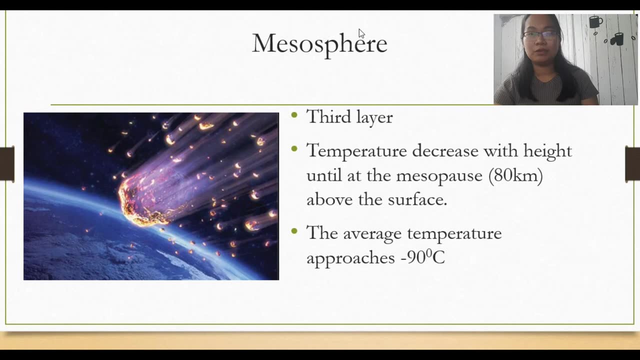 So we know that ozone layer absorbs energy or absorbs ultraviolet radiation. that's why the temperature increases at that particular layer of the Earth's atmosphere, The mesosphere. it is the third layer of the atmosphere. What happens here again, temperature decreases further from the Earth. 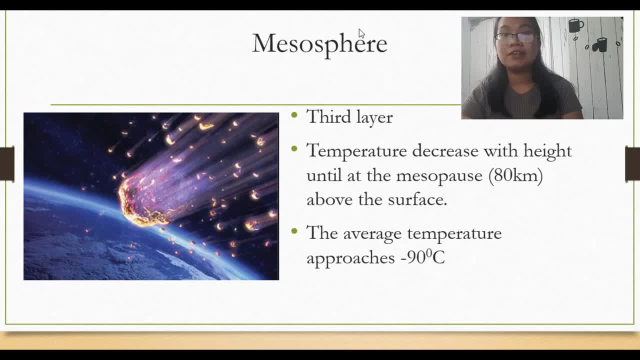 and also you are moving further from the Earth. This is called the stratosphere. The average temperature approaches at negative 90 degrees Celsius In the mesosphere. they say that the meteors reach there. based on that illustration, It is where meteors are destroyed in that layer. 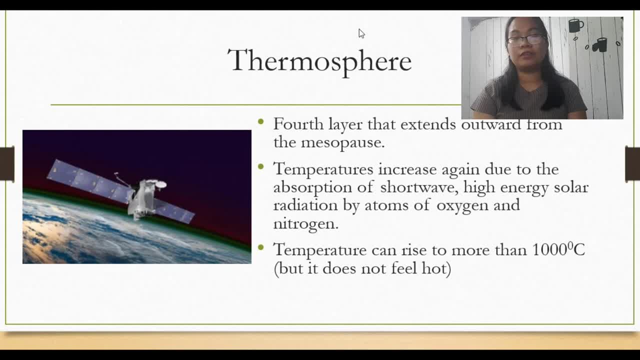 The thermosphere is the outermost layer of the atmosphere And then it expands outward from the mesopause. So that is the boundary of the mesosphere and thermosphere. Temperatures increase again due to the absorption of shortwave. When we say shortwave, they have high energy. 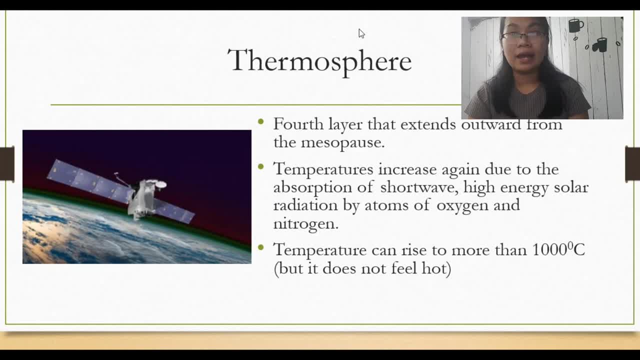 because they have higher frequency. They are high energy, solar radiation by atoms of oxygen and nitrogen. Temperature can also rise to more than 1000 degrees Celsius, but surprisingly, it will not feel hot. Why In the thermosphere its temperature is high. 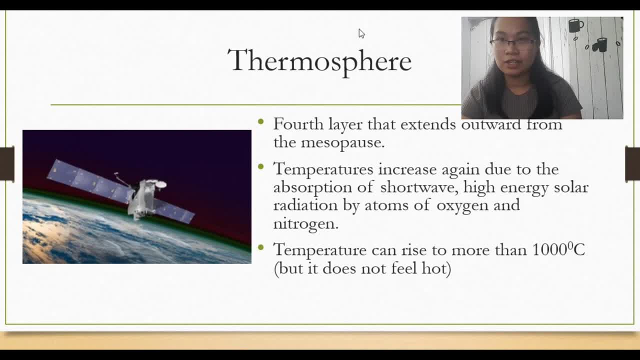 When we say temperature is the average kinetic energy of the translational motion of the particles, The movement of particles is fast, But take note, as you move higher the altitude the pressure decreases. When we say the pressure decreases, that means the particle spread set decreases. 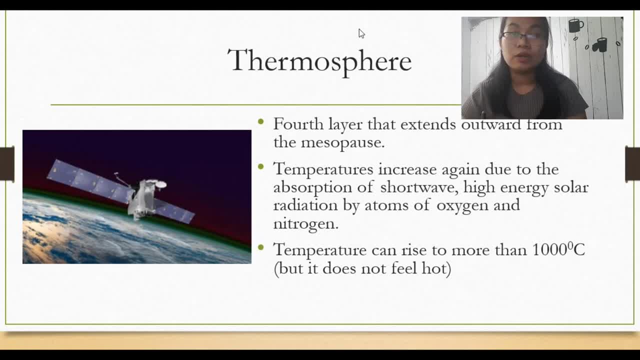 At a particular area or at a particular volume. So at that layer, even though the kinetic energy of the particles is high, the number of particles is considerably low, So it will not result to a significant amount of heat that we will feel hot. 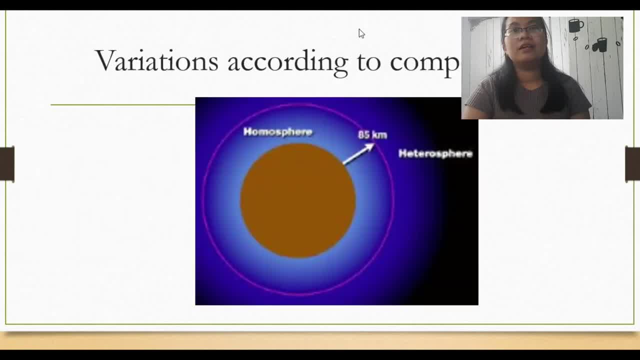 Okay, There is also another layering of the atmosphere that they consider because of composition. We have the homosphere and then the heterosphere. When we say homosphere, of course it means that the composition is uniform, from the term homo, from the term homogenous in chemistry. 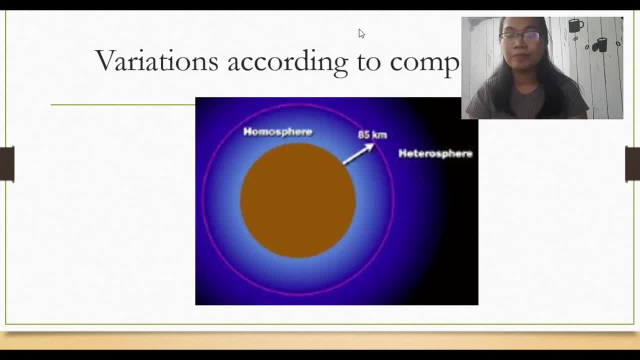 But when we say heterosphere, the proportions of the composition of gases are different, Unlike in the homosphere, the proportions of gases are uniform. First, in this one, the heaviest layer is nitrogen And then the lightest layer is hydrogen. 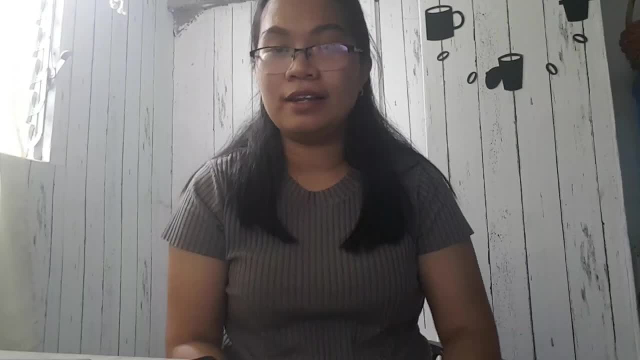 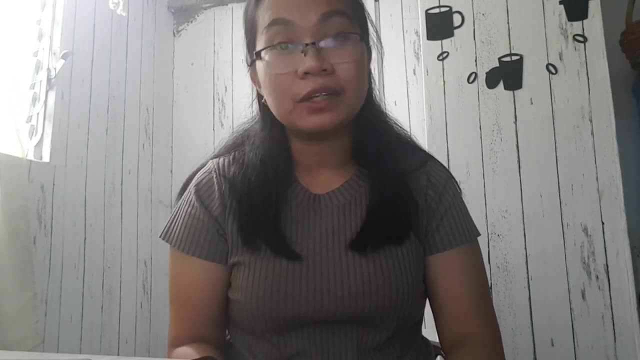 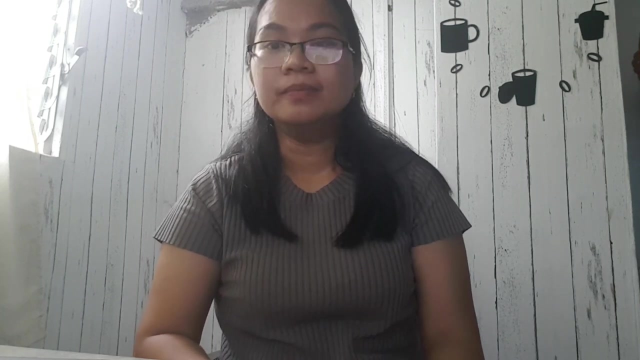 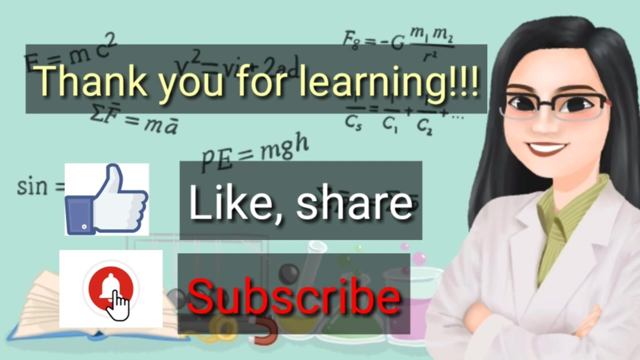 Okay, That is our discussion about the atmosphere and the different gases present in the atmosphere, which plays an important role in our weather conditions. In the next video, we are going to discuss about the heating of the earth. Okay, Bye. Subtitles by the Amaraorg community.